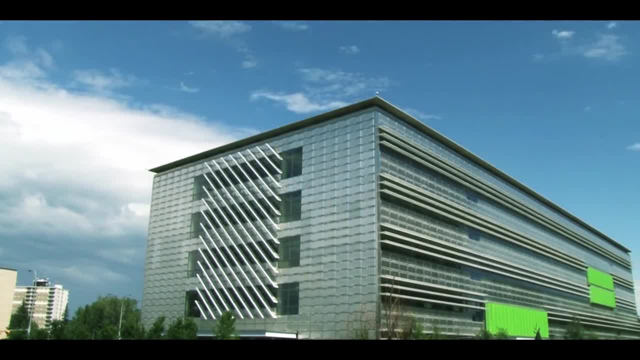 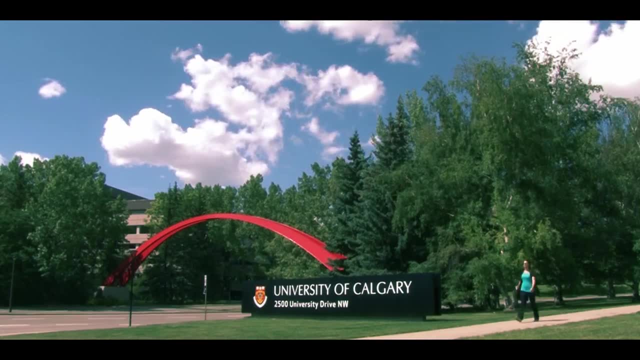 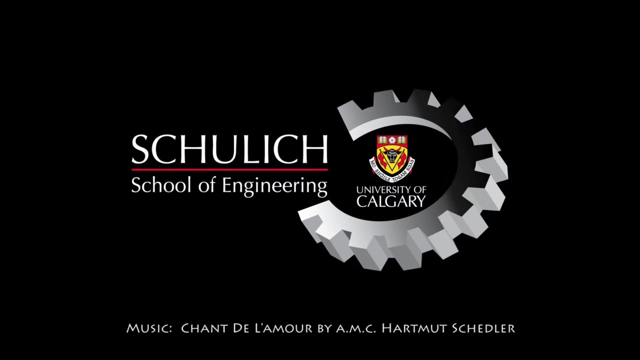 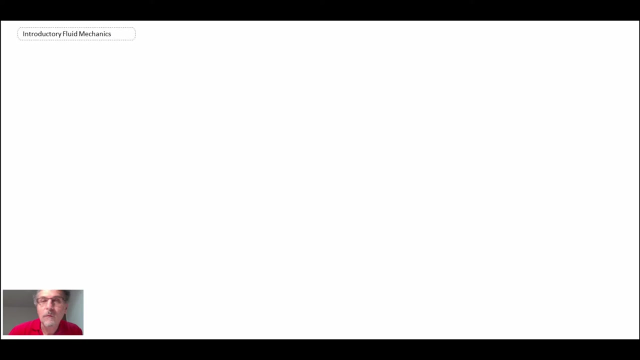 What we're going to do now is we're going to start the derivation for a stationary fluid, and that is the basic equation for fluid statics. And what we'll do: we'll begin with our coordinate system And we're going to consider a chunk of fluid. 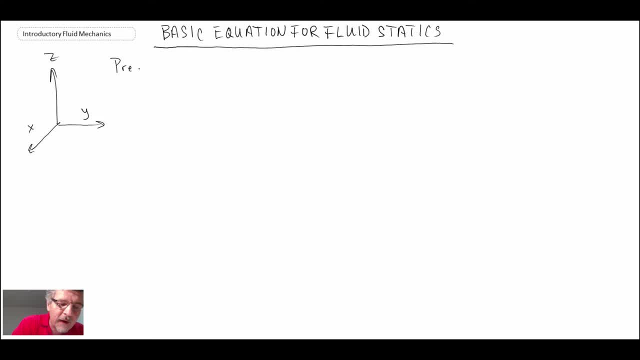 and we'll be looking at the pressure forces on that chunk of fluid. And so we have a chunk of fluid size dx, dy, dz, and we're going to assume that the pressure at the center is given by little p and we're going to assume that the pressure at the center 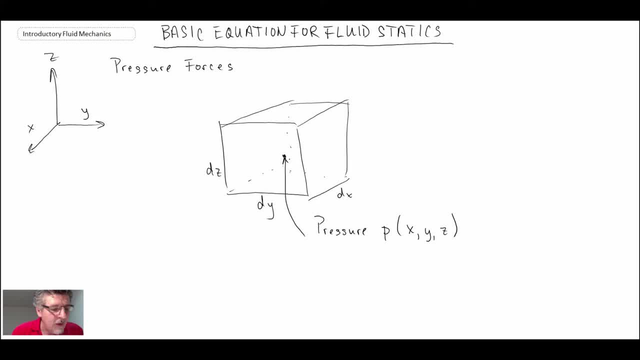 is given by little p at x, y and z. Now we're going to consider to begin with only the y component of pressure forces. but on the back surface there would be a pressure force and it would act like that, and on the front surface there would be another pressure force. 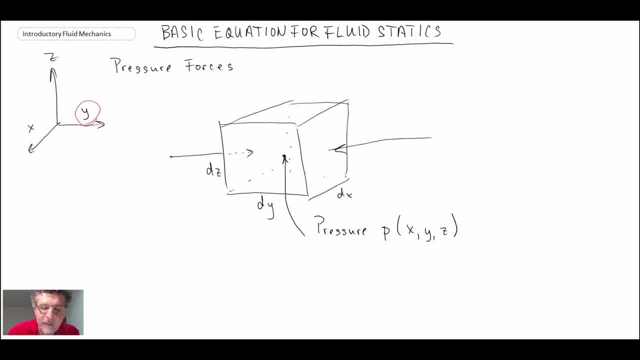 And remember, pressure, we said, acts normal to the surface, and so it would be acting inward into the chunk of fluid. So what I'm going to do, I'm going to use a Taylor series expansion in order to express sorry, to expand the pressure that would be on both of those two faces. 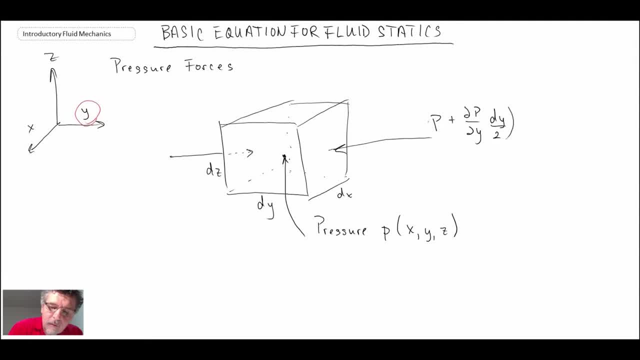 the left face and the right hand face. Okay, so there we have the pressures acting on the left hand surface and the right hand surface And, in case you're wondering, this came through a Taylor series expansion, and so I'll just do a little bit of a math aside now. 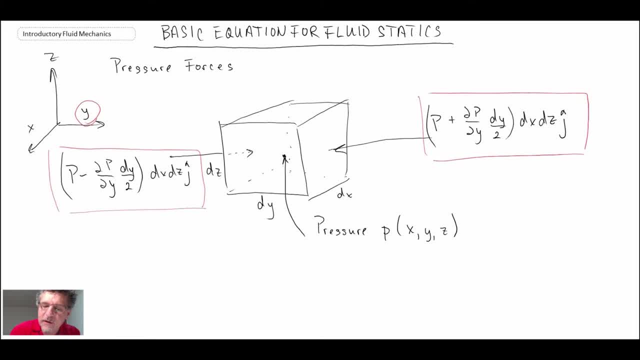 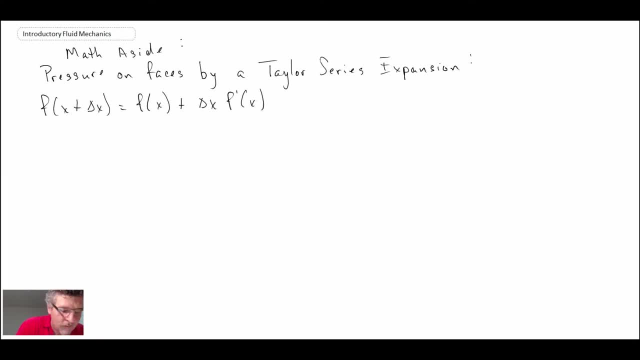 to explain where I was able to get those expansions or those terms for pressure. Okay, so there, what we've done is we've used the Taylor series expansion, and so here's the Taylor series expansion. 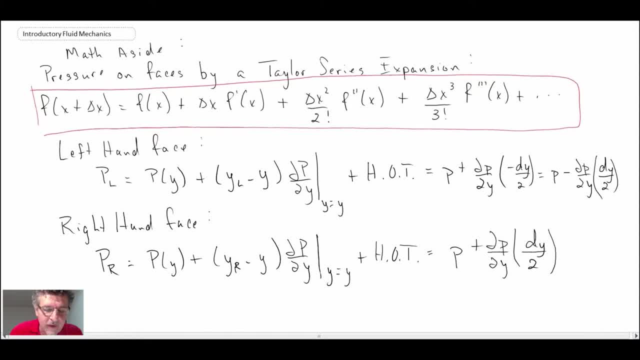 And we've done this for the left-hand surface and the right-hand surface, and so that's PL and PR, And what you can see is that we only go to the first derivative and then we have- these would be the higher order terms here, which would be second and third order. 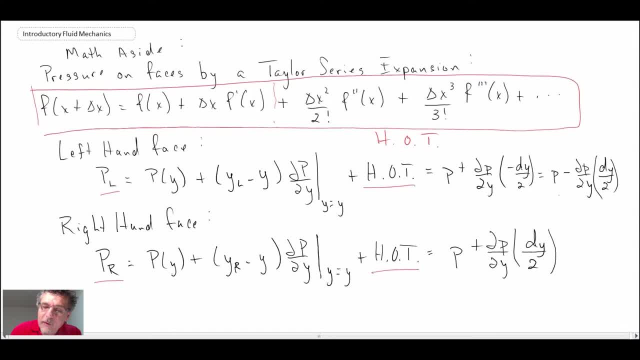 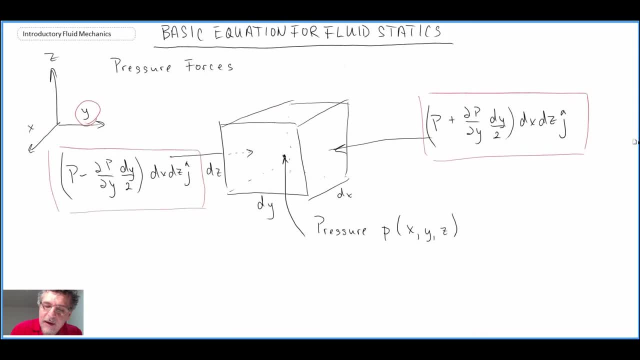 and we're neglecting those And with that we come up with an expression for the pressure on both the left-hand face and the right-hand face that if we look back you can see we have that within our expression for the pressure. 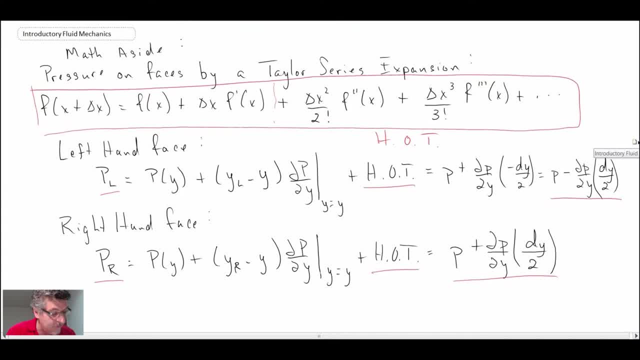 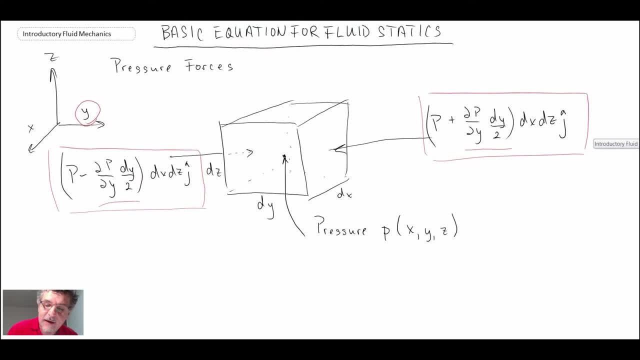 And in case you're wondering where the pressure came from, that is where it came from. So, with that, what we can do is we can continue in that method, and we've done that here for the left and the right in the Y direction. 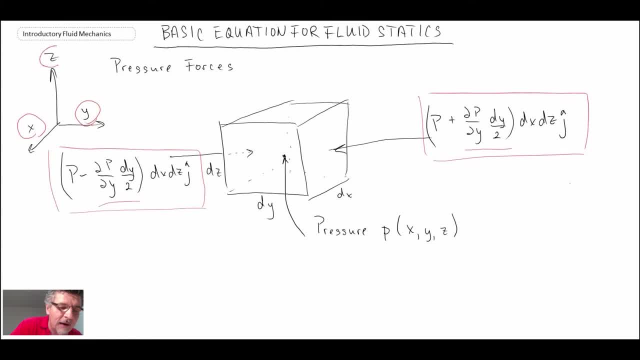 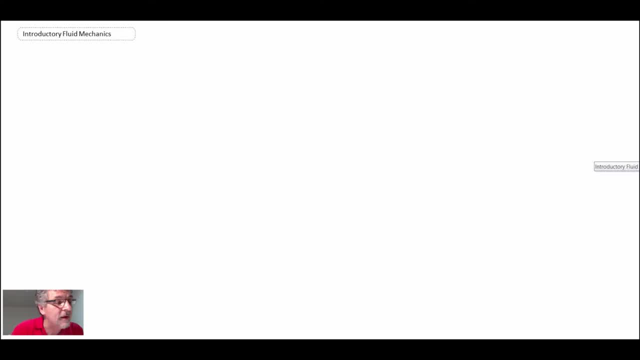 Now what we'll do? we continue on with the X and with the Z direction, and what we can do is rewrite or expand it for all three faces. So what we're going to do is we're going to write out the vector surface force due to pressure. 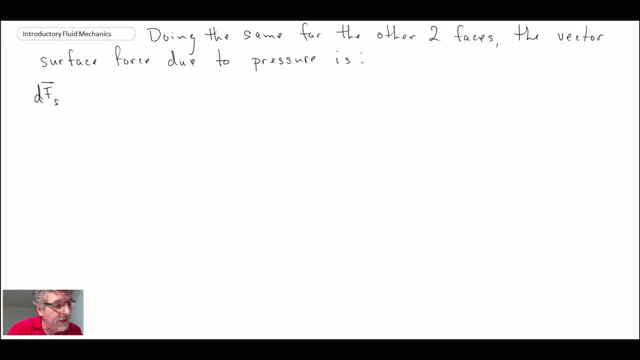 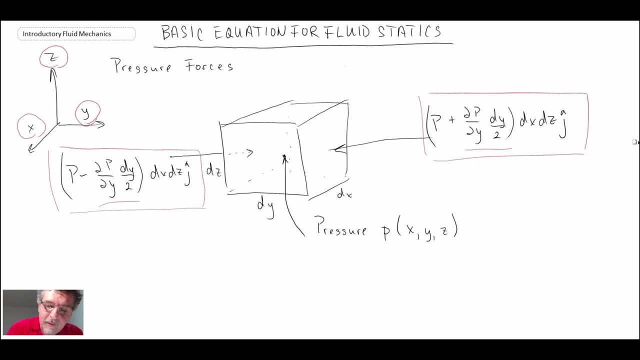 And we'll do this for the X direction, the Y and the Z, And for this we're multiplying by the area that the X direction pressure is acting on, which is dY, dZ, and then on the face, on the upper side, in in the x direction. let's go back to our cube of fluid. 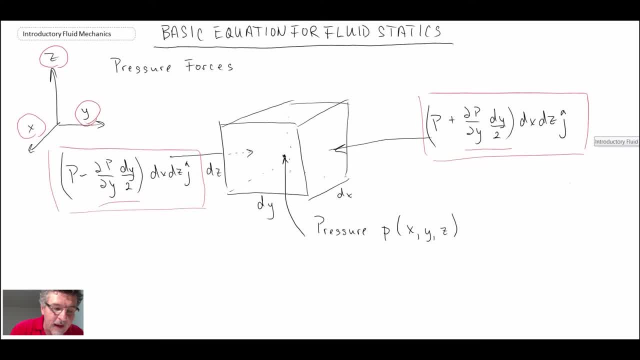 which was right here. so we're now dealing with the x direction. we said x was positive in this way. so the back face is back here. the front face is here, but notice that in this case we have the unit vector. is i in that direction? and here we're doing a dot product, but the unit 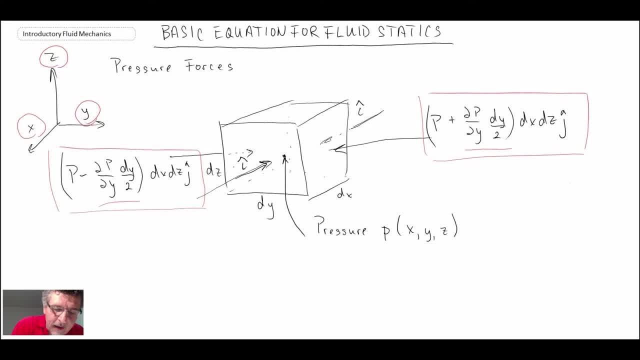 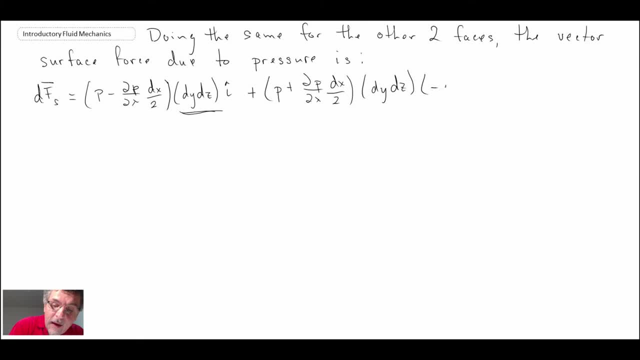 vector here is in the minus i direction and consequently we need to carry that through when we do our expansion. and so we have minus i for the unit vector and we'll do that for the other surfaces as well. so, okay, so we get that for the surface, the vector. surface force due to pressure. 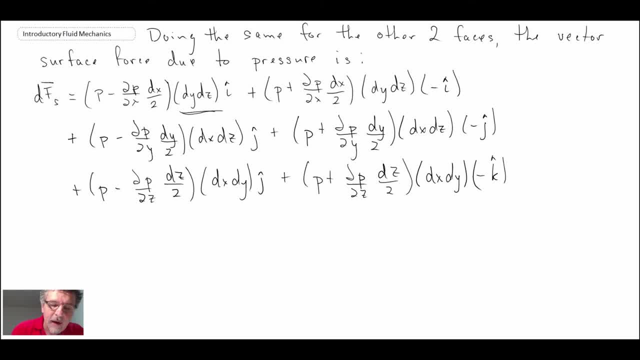 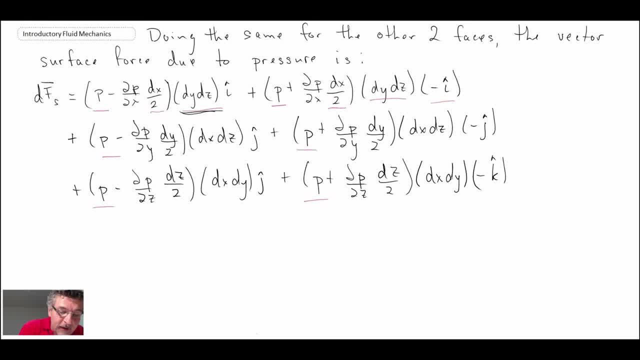 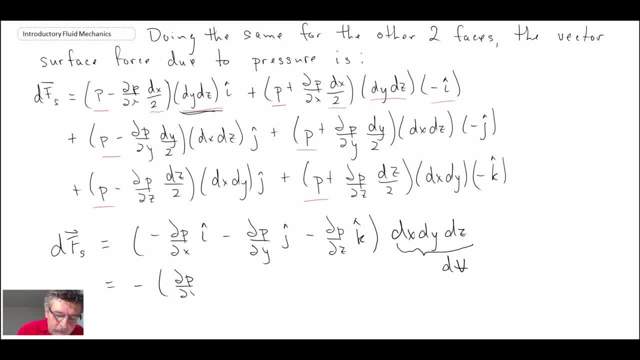 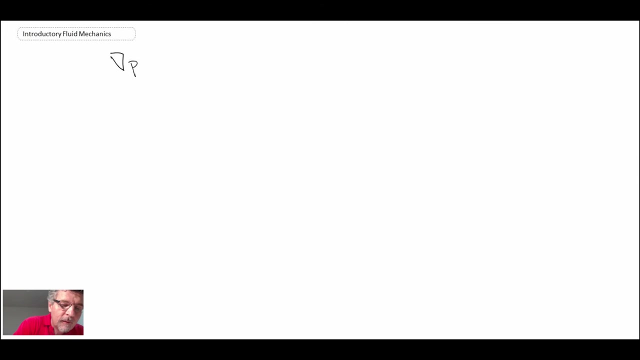 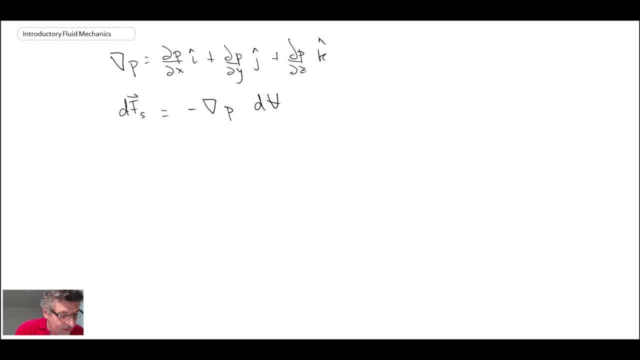 And then what I'm going to do. I'm going to divide both sides by dv and I'm going to move the minus sign over, So I'm going to have the gradient of P on the left and that will be equal to dfs by dv. 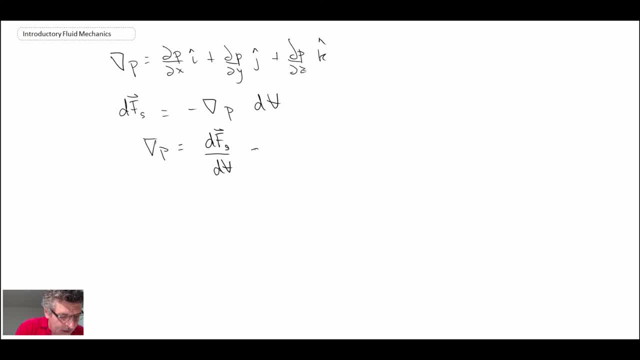 And I'm going to define this as a new force. I'll do it as a little f And, just like in thermodynamics, when you have intensive properties, that will be a little f, which will denote force per unit volume. So that is the equation, the beginning of the equation.